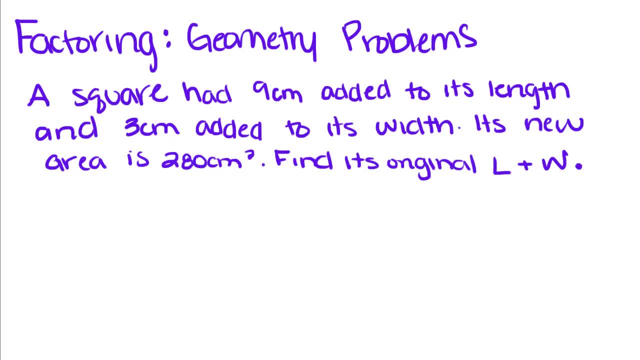 Okay, so today we're going to learn how to use factoring to solve geometry problems. So a square had 9 centimeters added to its length and 3 centimeters added to its width. Its new area is 280 centimeters squared. Find its original length and width. 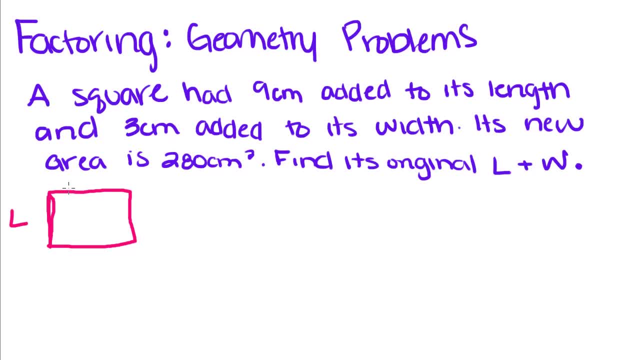 So first we had a square that had a length and width And now we have a new square whose length is L plus 9 and W plus 3 for its width. So we know that this new area is 280 centimeters squared. So to find area we multiply the length. 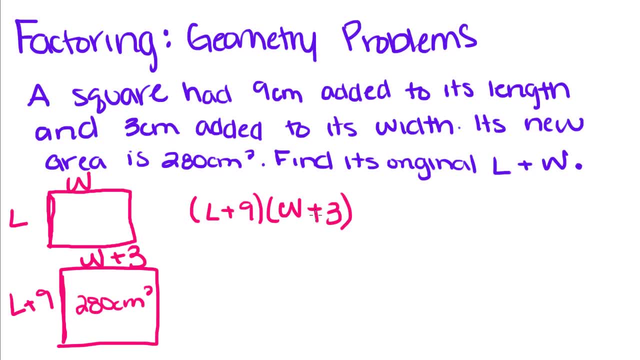 Okay, Okay Times the width to get 280.. And since it's a square, that means that this length and width are equal. So we're going to represent this with an X here and not an L, and an X here instead of a W. 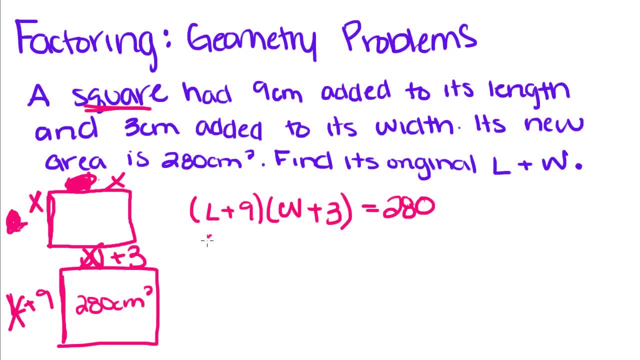 So this is X plus 9 and this is X plus 3.. So when we rewrite the area, we get X plus 9.. So X plus 9 plus X plus 3 equals 280.. Now we have to foil this out in order to set this equation equal to 0. 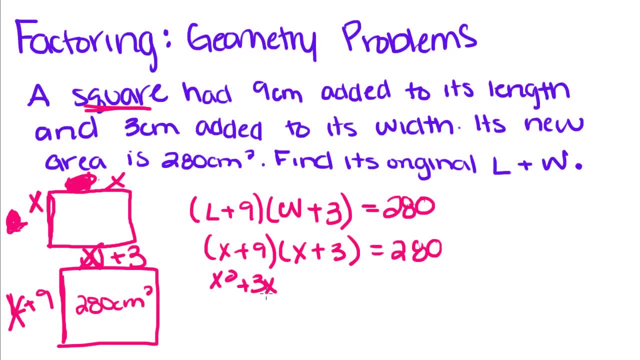 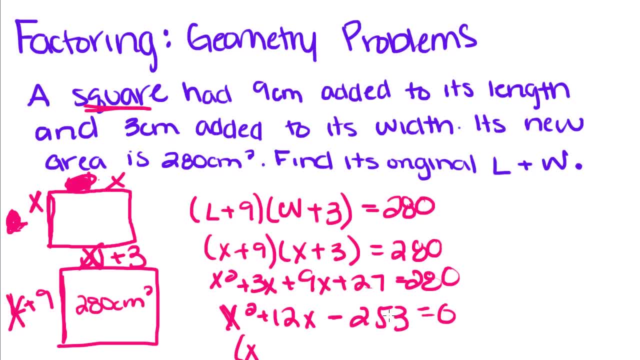 So we get X squared plus 12X minus 2Y. So we get X squared plus 12X minus 2Y. So we get this. so we get that 2 and 3 divided by 23 is 11, and 23 plus a negative 11 gives us 12.. 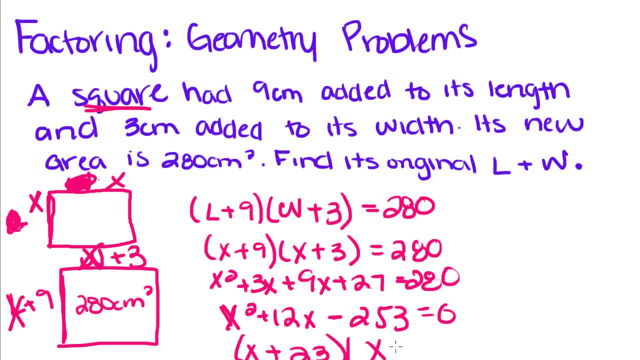 So that's so. we know that a positive 23 and a negative 11 are going to go there. So now we set each one of these equal to 0. If you subtract over, you get X equals the negative 23.. And we know that a 20, which is 25, is 0. And we know that a 20, which is 25, is 0. If you subtract over, you get X equals negative 23.. And you know that a 22 is 0. And if you add this over, you get x equals 11.. 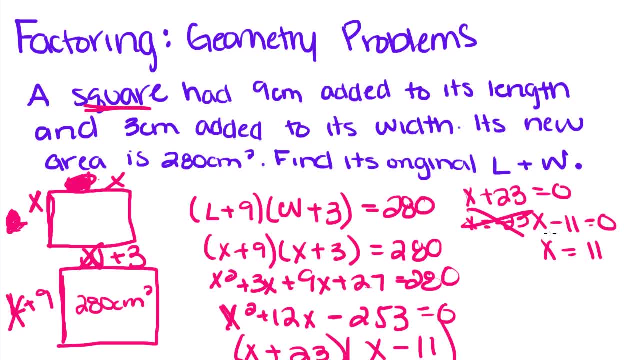 Since we're talking about distance, we can kick out this answer, because distance can't be negative. So we find that x is equal to 11.. But they wanted to know what the original length and width was. So that means that its original length is 11,. 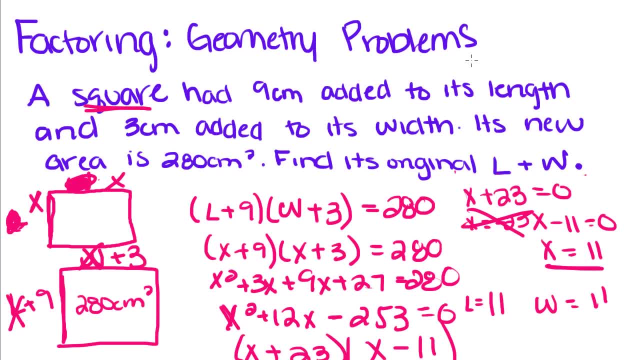 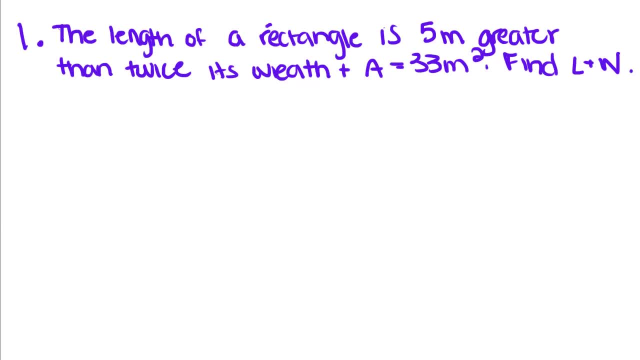 and its original width is 11.. Let's do another example. The length of a rectangle is 5 meters, greater than twice its width, And its area is equal to 33 meters squared. Find the rectangle's length and width. So the length of a rectangle is 11.. 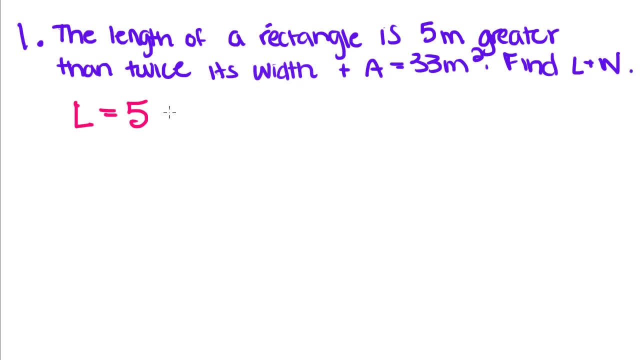 And its angle is 5 meters greater, so 5 plus twice its width, So 5 plus 2w. So its width is going to be equal to just plain w. So its area is equal to 33 meters squared. So that means that its width is equal to 33 meters squared. 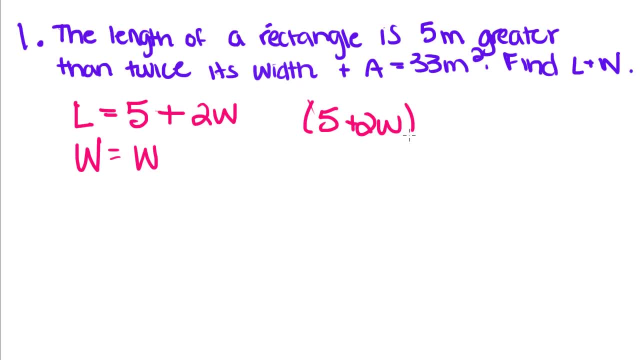 So that means that its area is equal to 33 meters squared. So that means that its length times its width is equal to 33.. If we distribute this w, we get 5w plus 2w squared equals 33.. Now we're going to set this equation equal to 0..